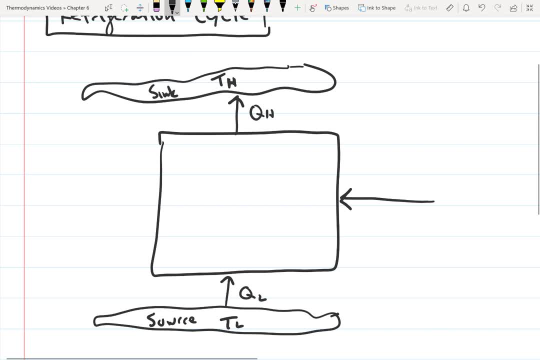 And this is Q high, And this is the heat that's being rejected to the room. And then, in order to move that heat, basically we're moving heat from a low temperature source to a high temperature source, which isn't going to just happen on its own because, remember, heat. 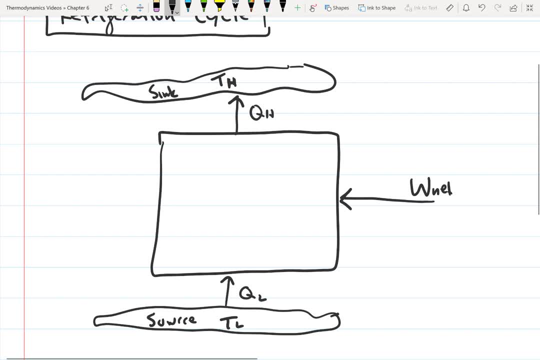 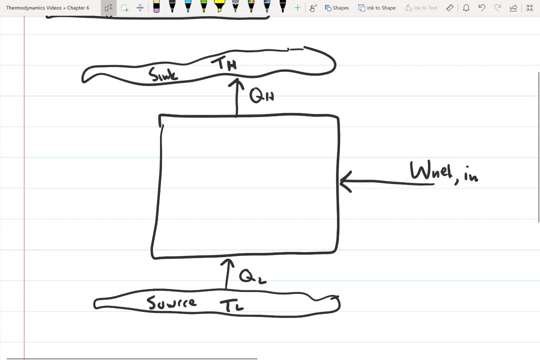 will transfer from high temperature to low temperature. So if we want to do that in the opposite way, we need to input work. So we have some work in, And so let's look at what we actually have in here. So, first of all, right here. so let's just 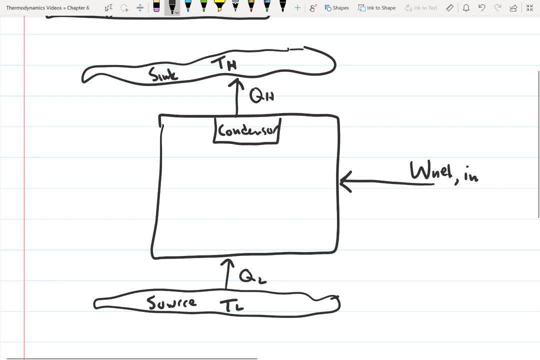 start here. So we have a condenser. The fluid inside this condenser is going to be basically condensing and heat is going to be removed from the fluid And, like the heat engine, we still have a working fluid flowing through our cycle And in a refrigerator, this working. 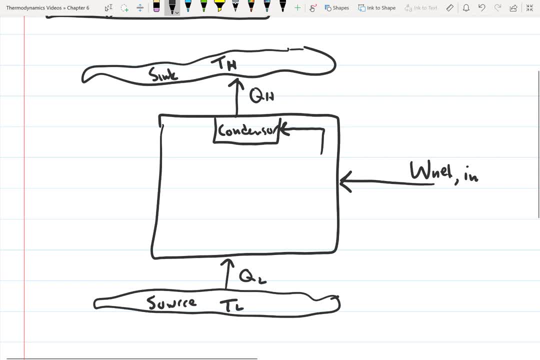 fluid is normally some kind of refrigerant. So we have the condenser. Right here we have a compressor, So this is the compressor, And then fluid is going to flow into the compressor from the. so right here we have an evaporator, And this is the evaporator, is really technically just a. 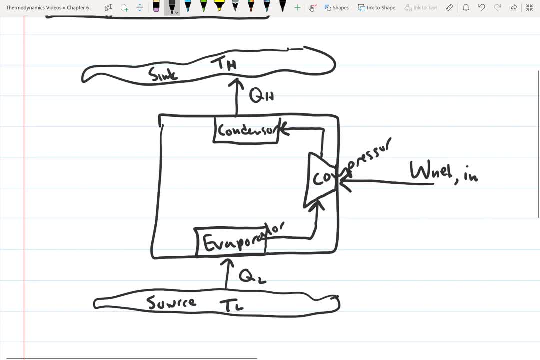 boiler, But in a, in a refrigeration cycle, it's called the evaporator. And then right here, so before the evaporator, we have a throttle, So the fluid flows from the condenser to the throttle. So what the throttle is doing is it's reducing. So when the the fluid goes through the 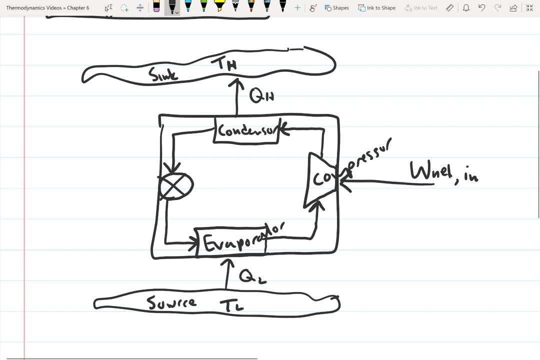 condenser, it's at high pressure. It gets to the throttle. The throttle is going to decrease the pressure Of the fluid to the pressure of the evaporator, because the evaporator is going to have a lower pressure than the, than the condenser and this evaporator, So the fluid is going to 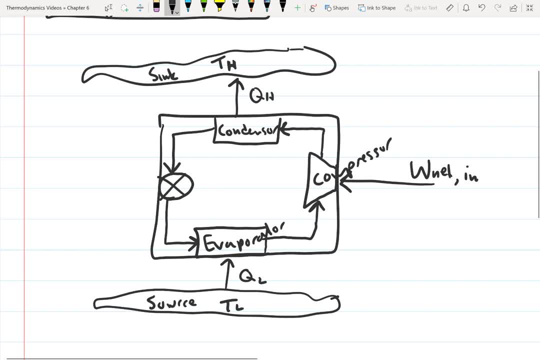 so the throttle is going to drop the pressure of the fluid or the refrigerant. the refrigerant is going to go into the evaporator. The evaporator is going to turn the liquid into vapor, And in order for the liquid to be turned into vapor, it needs heat. And 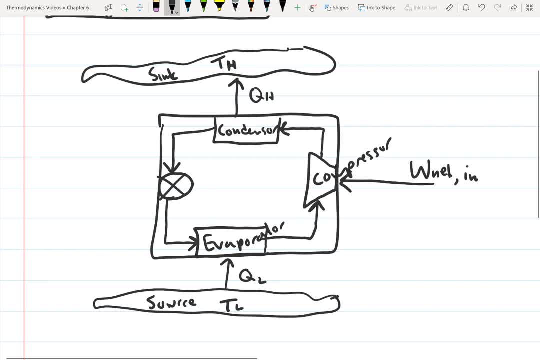 so it's going to remove the evaporator, is going to remove heat from whatever we're trying to cool. So this might be the inside of the refrigerator And it's going to use that heat to turn the refrigerant from a liquid into a vapor. And then this, this fluid, is going to go from the 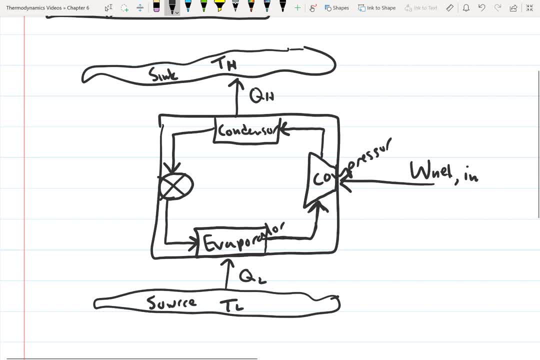 evaporator into the compressor. The compressor is going to compress the fluid, So it's going to be raising the pressure of the fluid, And when it does that, it's also going to. it's also going to be increasing the temperature of the fluid, And so the temperature of the fluid is going to be. 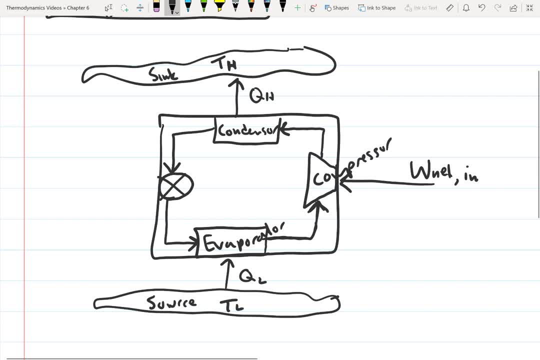 increased to a temperature higher than the heat sink. So it's going to be. the compressor will be increasing the temperature of the fluid to a temperature that's higher than than T high, And so then when the fluid gets to the condenser, it's at a higher temperature than T high. 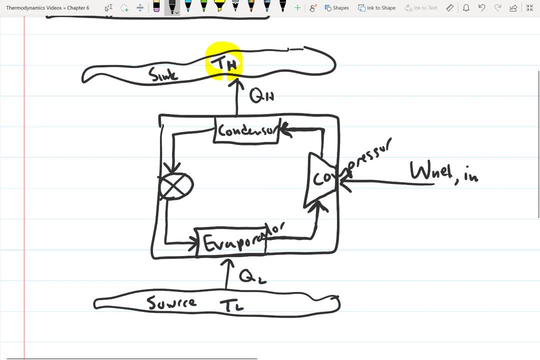 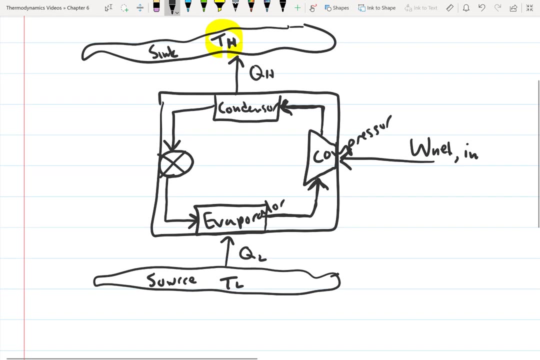 And so it's going to lose heat to the, to the sink, And And the fluid's going to flow through the condenser back out to the throttle and the cycle is going to continue And typically in a refrigeration cycle we're going to be using some sort of refrigerant. 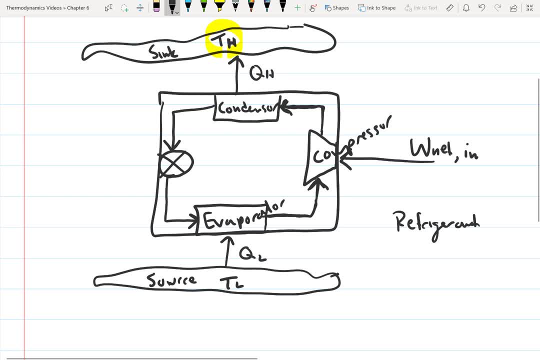 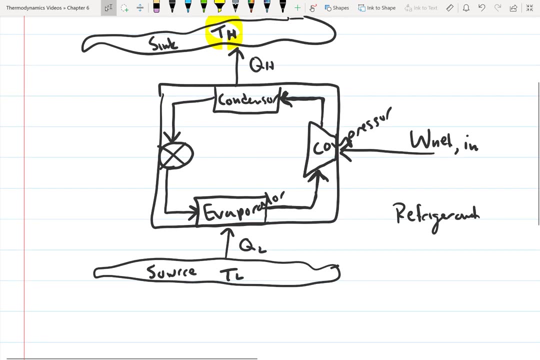 So what we want to do is figure out. we want to basically do the same thing we were doing with the heat engine. So with the heat engine, we calculated what the highest efficiency was that we could have. In the case of the refrigeration cycle, we're going to be calculating something similar to the efficiency, but it's not actually going to be called efficiency. 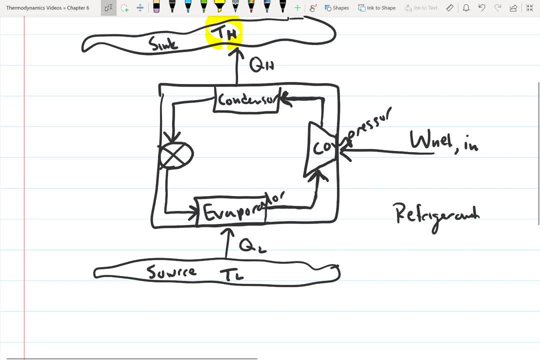 It's going to be called the coefficient of performance. So one difference between the refrigeration process versus, say, a heat engine process is: with the heat engine we couldn't get more work than heat that we put in. It would always be less. 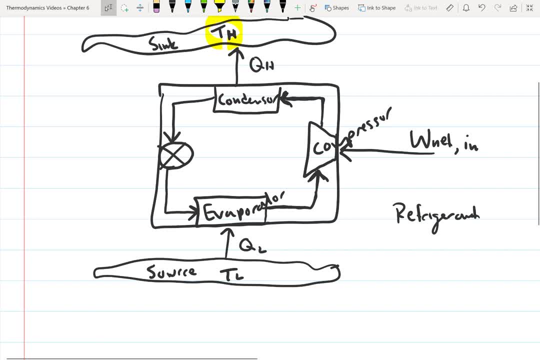 Our work is always going to be less than the heat we put in, and that's because we had to have a certain amount of heat rejected. With the refrigeration cycle we can actually remove more heat than so. more heat can be removed from the refrigerated space than the work input. 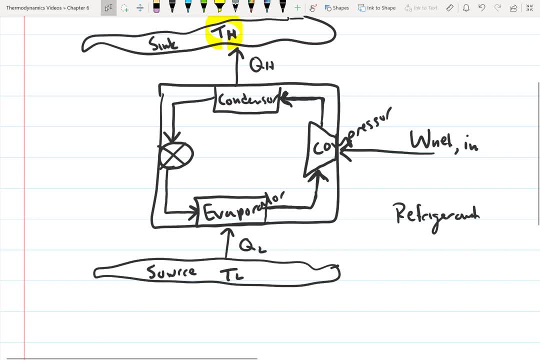 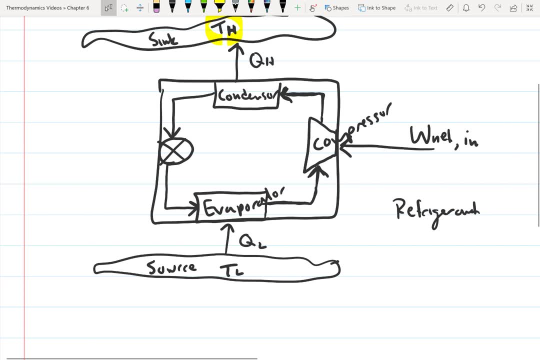 So the heat removed can be greater than the work input. So basically we end up with: if we were to calculate our efficiency the same way that we calculate the thermal efficiency, this we can end up with a value greater than one. 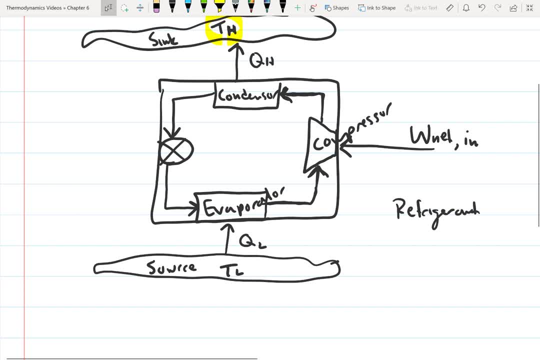 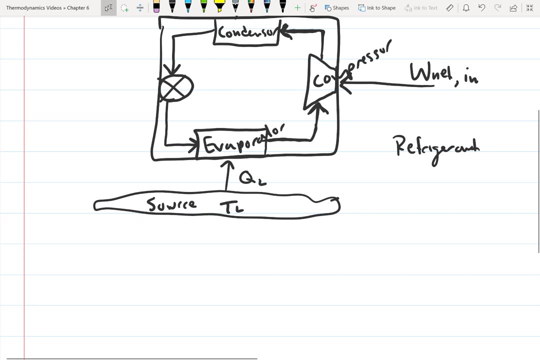 And so for a refrigeration cycle, the term coefficient of performance is used instead of a thermal efficiency, because it can be greater than one and you can't have a thermal efficiency that's greater than one. So let's go ahead and look at this. 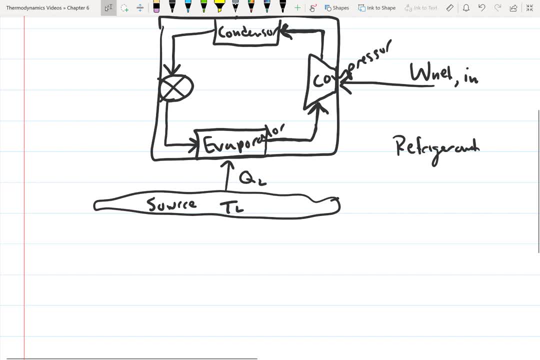 So we want to calculate what's called the coefficient. So what we want to do is calculate what's called the coefficient of performance, And this is going to be equal to the desired output over the required input, And so the desired output is just simply the heat transfer of interest. 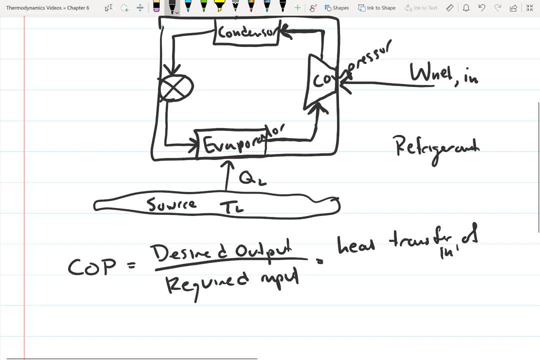 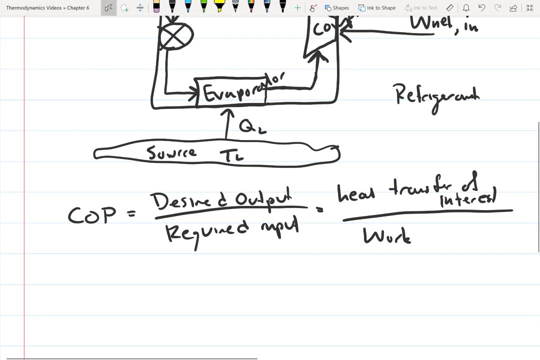 So this is the heat transfer of interest over the required input, which is the work. so the the work that we have to input into the system in order to transfer that heat. before we go further with this, we need to. there are actually two different refrigeration cycles that we can. 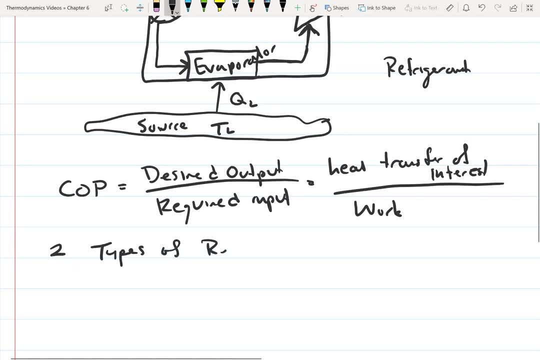 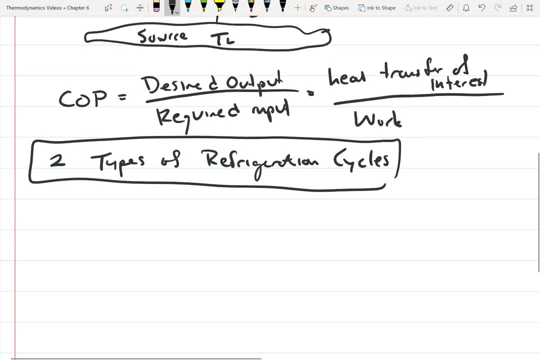 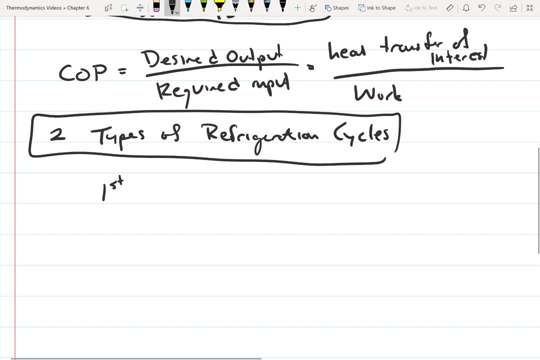 that we need to consider. so there are two types of refrigeration cycles, so we're going to consider the first one and then we'll we'll do the second one. so the first one is what we would typically think of as like a refrigerator, so i'm just going to put the first one. this would be like a. 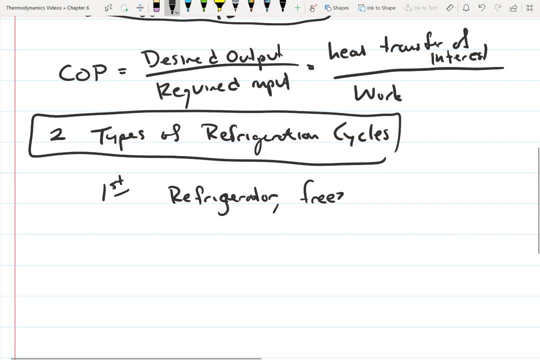 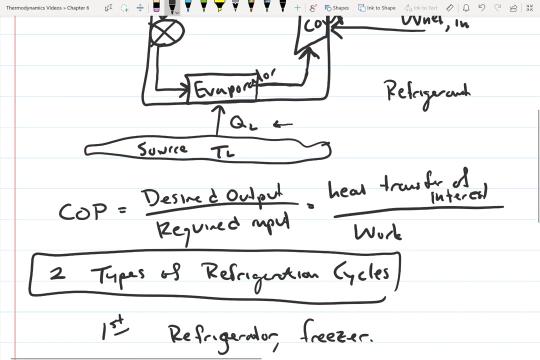 refrigerator or a freezer. so these are what you typically, typically have in your house, and so the coefficient of performance for a refrigerator or a freezer is: has this um subscript r to represent that that's a refrigerator or freezer? so the heat transfer of interest is q: l, so it's the heat that we're. 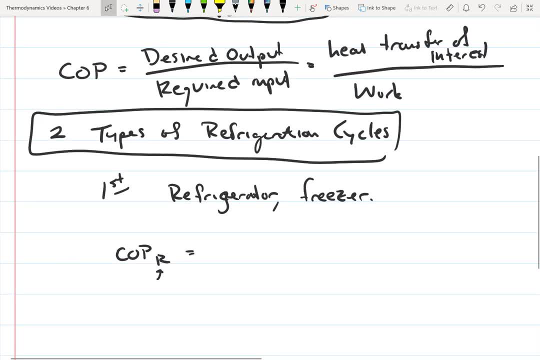 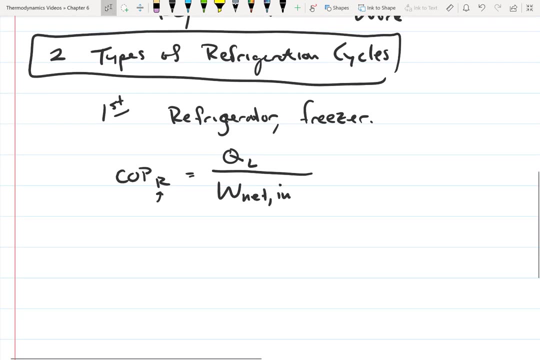 removing from the refrigerated space. so q l the heat transfer of interest is q l over, and then our required works. this would be the work net in. so what we want to do is basically, we're going to do the same thing we did for the, for the 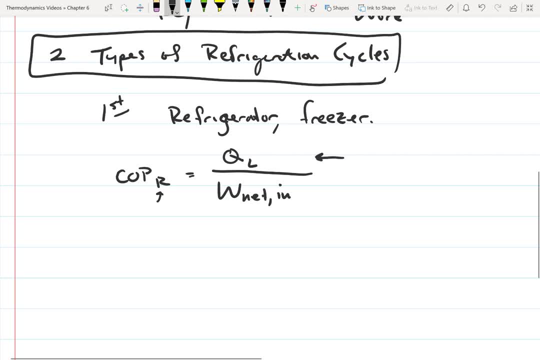 for the heat engine. we, so we know q l. what we want to do is calculate what the work net in is, and we're going to do that with an energy balance. so we have the work is equal to. so we're going to integrate over the cycle and remember this. so, since we have a cycle, du, so the change in the 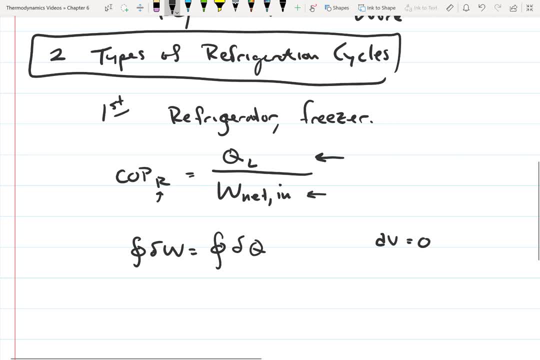 internal energy is equal to zero. because if we integrate over the entire cycle, like if we consider our cycle, so let's say this is a pv diagram. so if we have a cycle, we're ending, we're beginning and ending at the same state, so let's say that one is our. 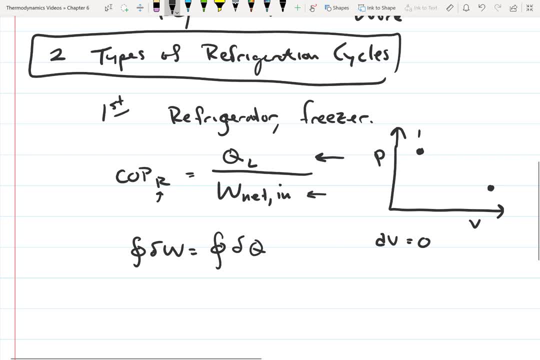 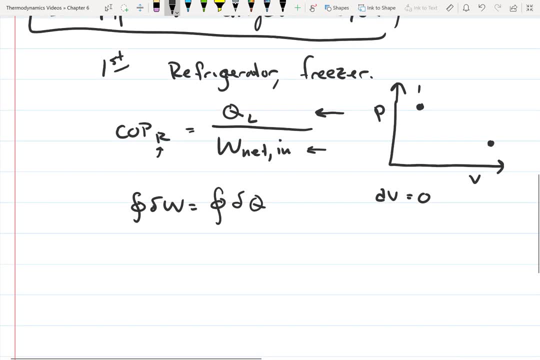 beginning state. if we have a cycle, we're beginning and ending at state one, because we're beginning and ending at the same state. so du is zero, um, so we have the, so we have this expression for that relates our work and heat transfer. if we, if we go over the entire cycle, first of all we have 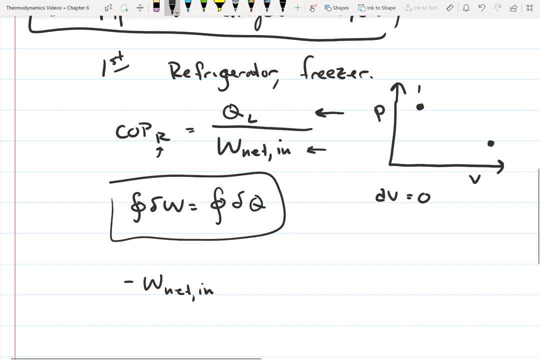 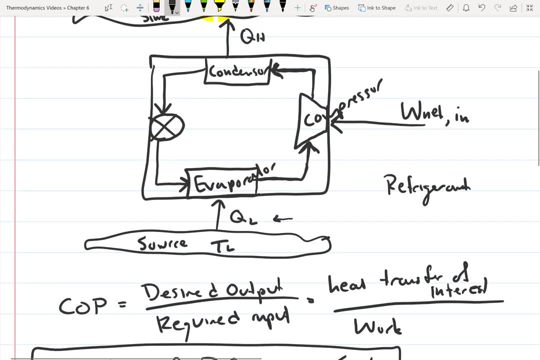 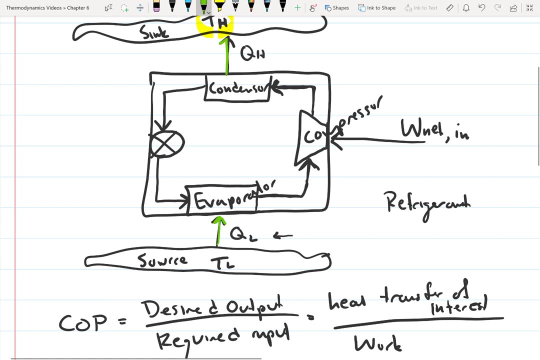 some work. net in the work is in, so we have a. so it's negative. and this is equal to, if we look at our cycle. so we have q l- heat transferred in. so q l is the heat transferred in and q h as heat transferred out. so we're going to have 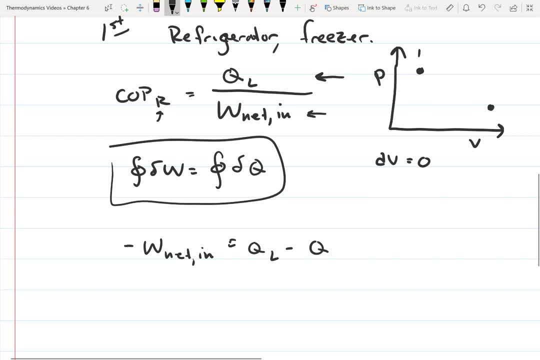 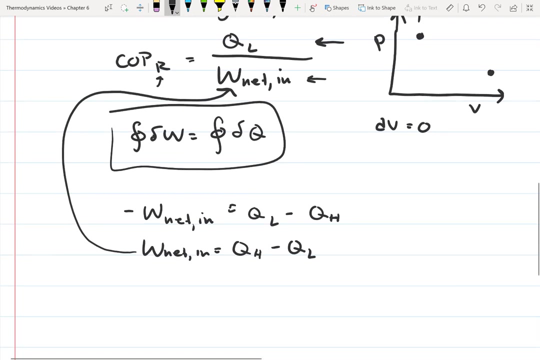 Q L minus Q H. and so then, if we multiply through the negative sign, we just get that the work net in is equal to Q H minus Q L. so what we're going to do is plug this work net into our coefficient of performance equation so we can write: 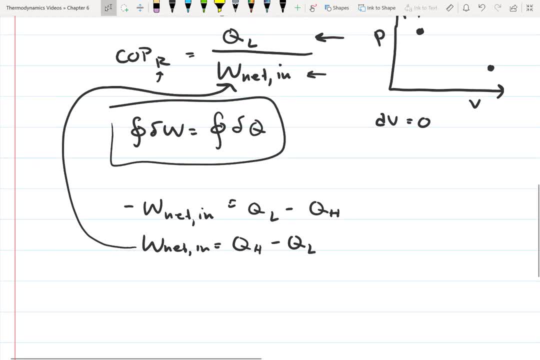 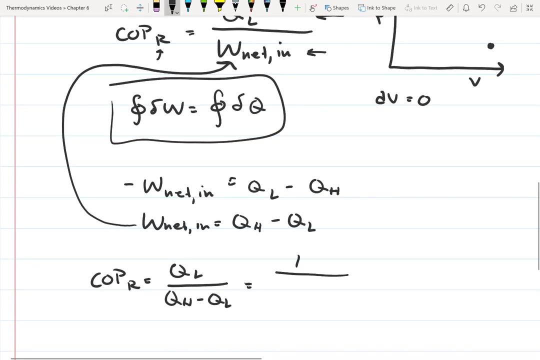 our coefficient of performance in terms of heat added and heat removed. so then the coefficient of performance for the refrigeration cycle is equal to Q L over Q H minus Q L. and then we can divide through. I'm going to divide through the Q L. so if we do that we get 1 divided by Q H divided by Q L. 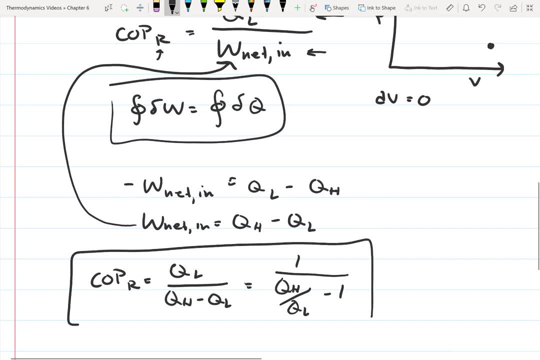 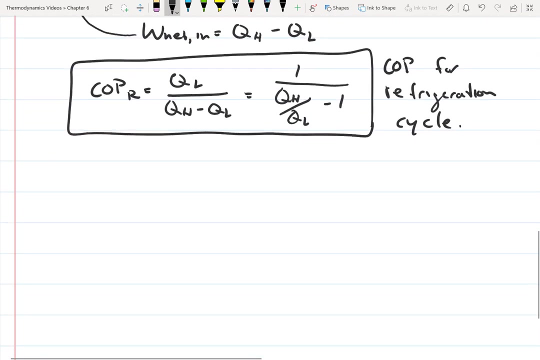 a- I'll fucking move this人- minus 1, so this is the coefficient of performance for the refrigeration cycle. so this is the COP for refrigeration cycle and remember this could be referring to like a freezer as well. the second, so the second refrigeration cycle. 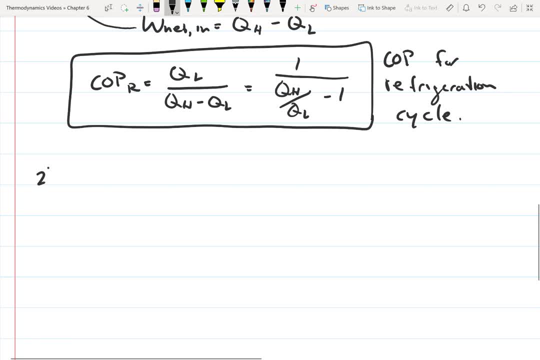 that we want to consider is for a heat pump. so I'm just gonna put that this is the second refrigeration cycle and this is for a heat pump and a heat pump. one thing that I want to make sure that's clear is that a heat pump is not a heat. 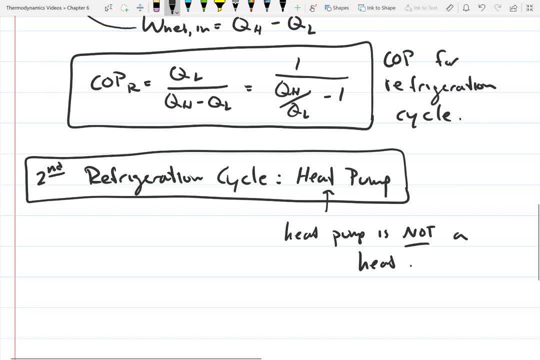 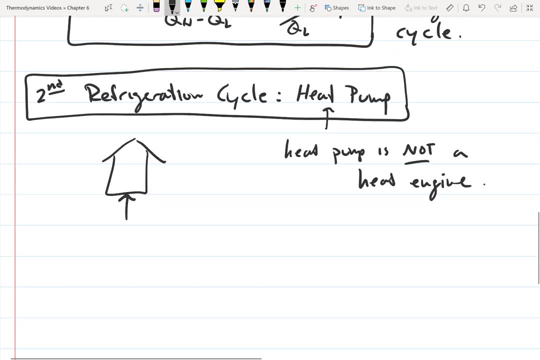 engine. so a heat pump is not a heat engine. so what a heat pump does is it really heats up a space that you're trying to take, that you're trying to keep warm, so it takes heat out of the cold outside air. so let's say you're heating your house so you're going to have some heat added to your 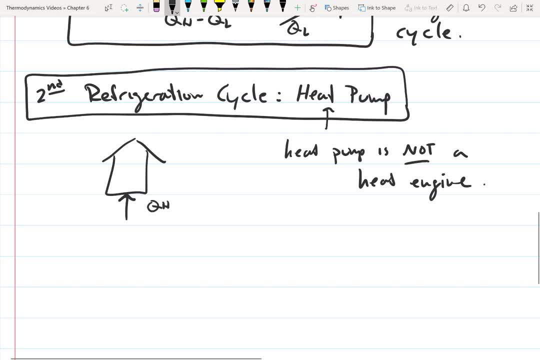 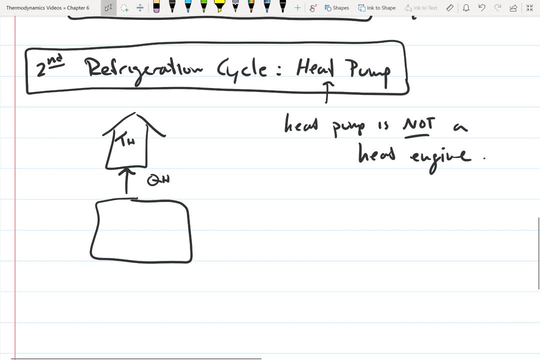 house. this is Q high and this might be at some high temperature and we have our cycle, so our heat pump cycle, and we're taking heat from outside. so this is our, this is our heat source and this is some T low and so we have Q low, so we're taking heat out of the cold. 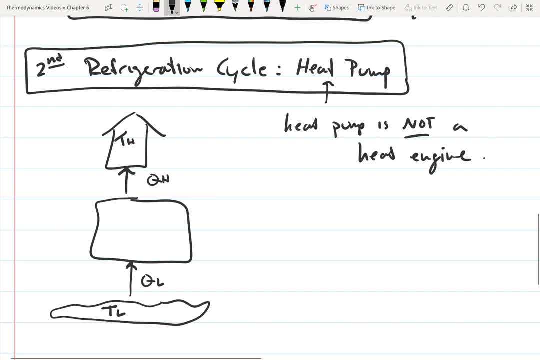 outside air and we're moving that heat into the house and this requires some work in. so this is often going to be some sort of electrical work that you're using to run your heat pump. so there's going to be work net in and you're going. 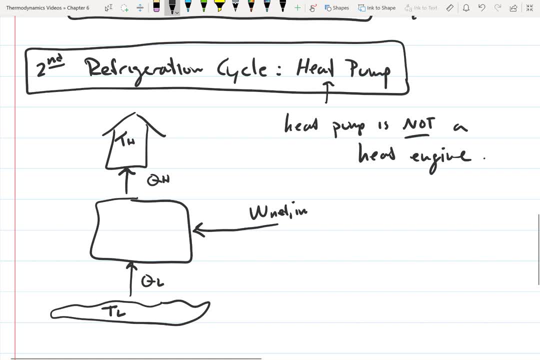 to be taking heat out of the cold outside and moving it into your house, and this heat pump will still have the basically the same components as a refrigeration cycle. so you're going to have a compressor, this is our compressor, and we have a condenser here. so condenser, an evaporator, and remember. 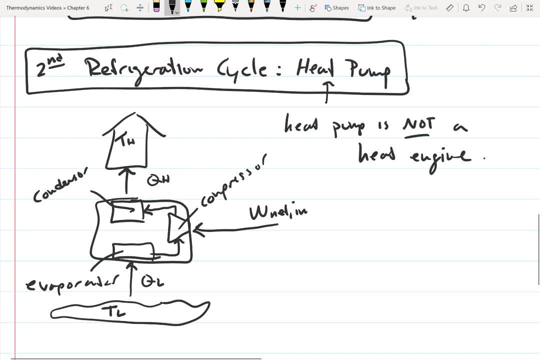 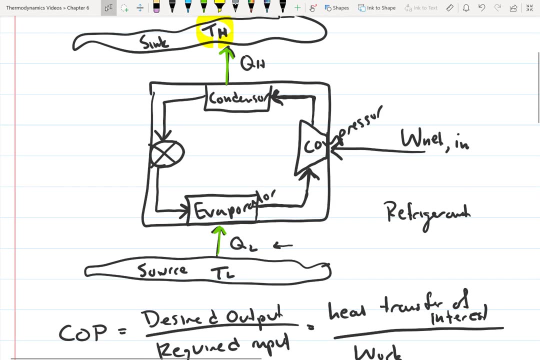 this is just like a boiler, but in a refrigeration cycle it's called an evaporator. we have a throttle, and so this is basically the same cycle that we considered for the refrigerator. it's basically a refrigeration cycle. the main difference is is that the heat 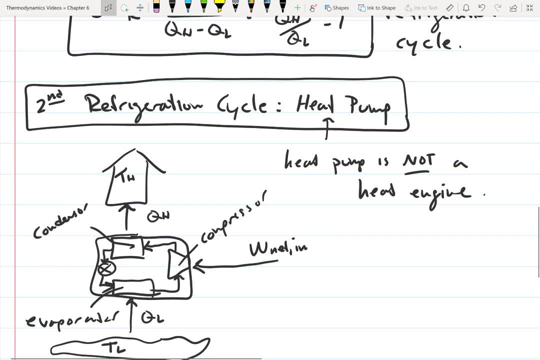 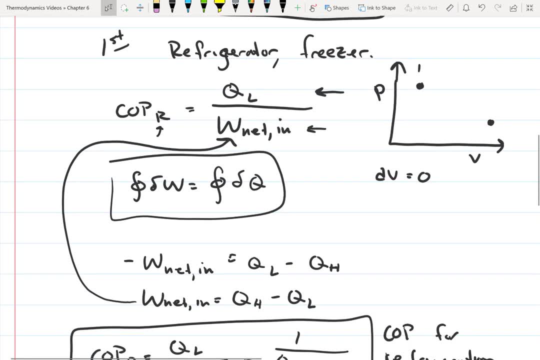 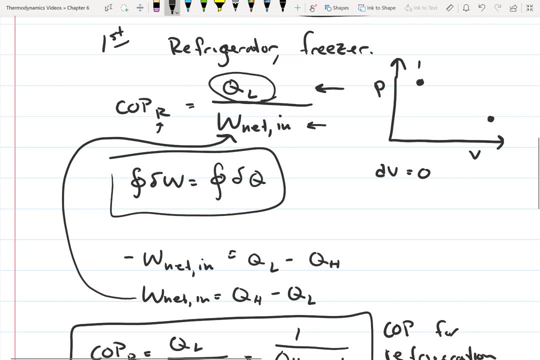 transfer that we're interested in a slightly different. so with the refrigerator, the heat transfer that like, if we go back up here, so when we calculate the coefficient of performance, the heat transfer that we were interested in was the heat that was being removed from the refrigerated space, so the heat that we're taking out of the refrigerated. 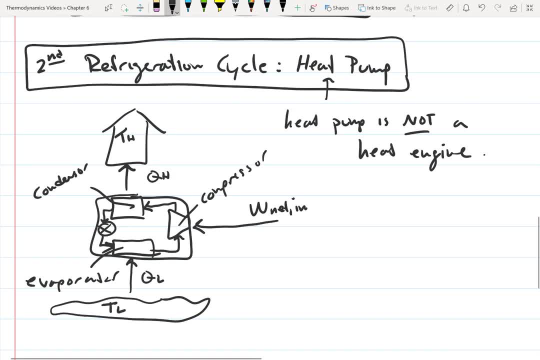 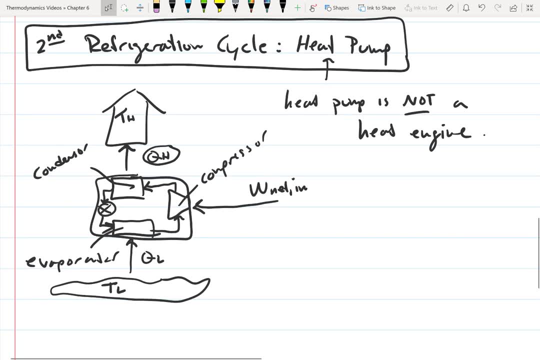 space, the with the heat pump, the heat that we're interested in is the heat that's being transferred to the house. so the heat that we're interested in is the heat that we're, that we're adding to the house to heat the house, and so the 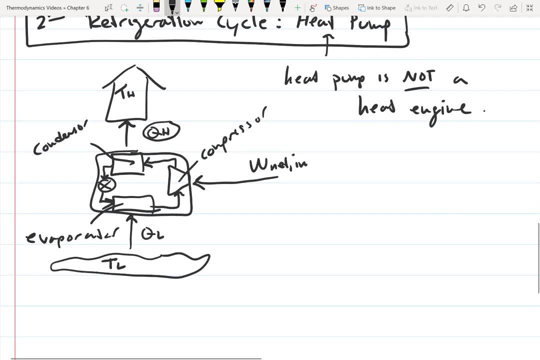 coefficient of performance for the heat pump is calculated slightly differently, so the coefficient of performance for the heat pump is. so, once again we have our heat transfer of interest divided by the required work in, and this time the heat transfer that we're interested in is the heat that we're transferring into. 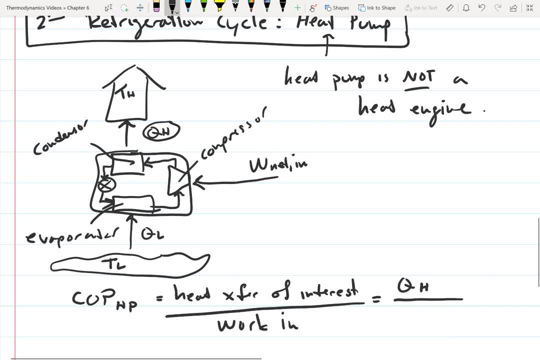 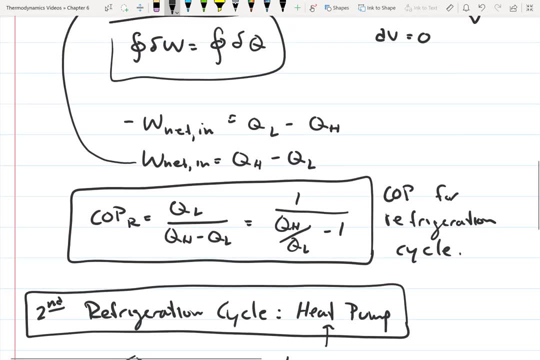 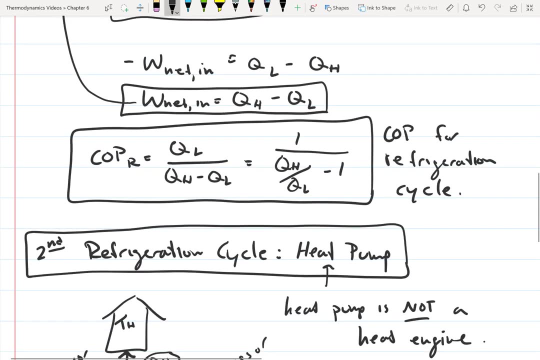 the house. so we're interested in Q high over the network in. the network in is going to be the same as the first refrigeration process. so the work net in is Q high over Q low. so we're just going to use that again and if you go through, 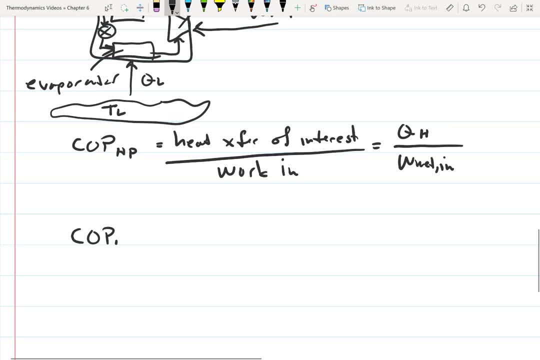 an energy balance. you can verify that. so the coefficient of performance for the heat pump is equal to Q high over Q high, minus Q low, and if we divide through the Q high, this is equal to one over Q low. and if we divide through the Q high, this is equal to one over Q low, and if we divide through the Q high, this is equal to one over. 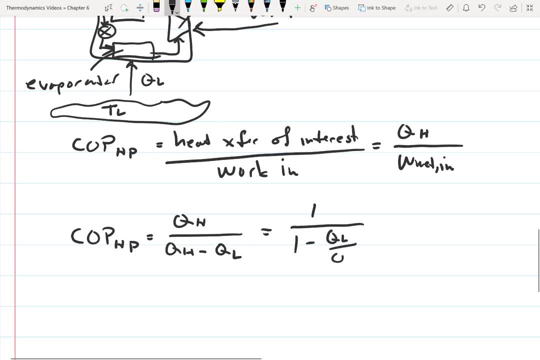 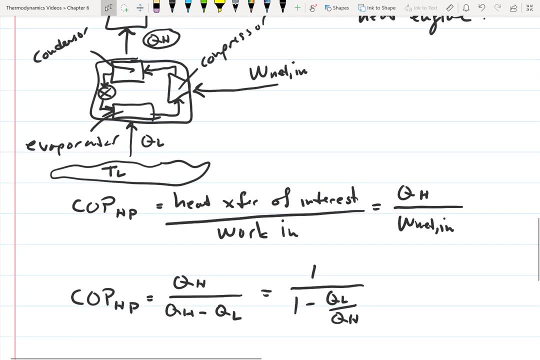 one minus Q L over Q high. so the main difference between the coefficient of performance for the heat pump and the coefficient of performance for the refrigerator is the heat transfer of interest is different. so this is the coefficient of performance for the heat pumps. this is the COP for a heat pump. so 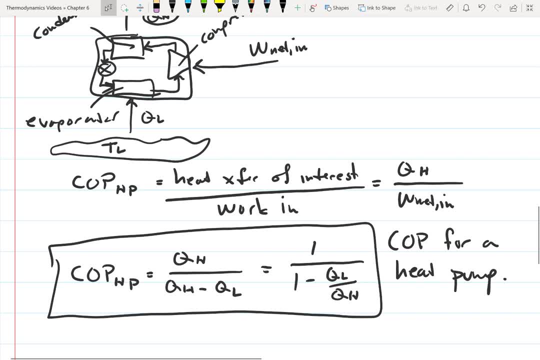 then we can treat our, our refrigeration cycle, or so our refrigerator or heat pump kind of. so we want to do the same sort of treatment that we did with the heat engine. with the heat engine, remember, we calculated the maximum efficiency that we could have for a heat engine and that was for the Carnot cycle- we can do the same. 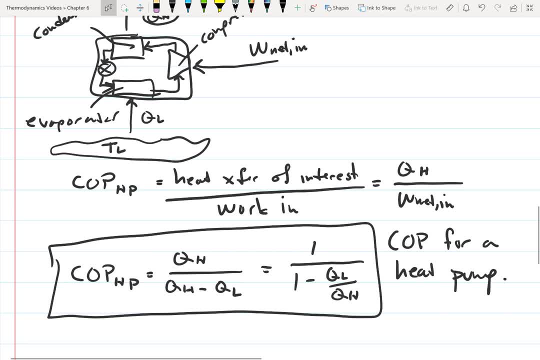 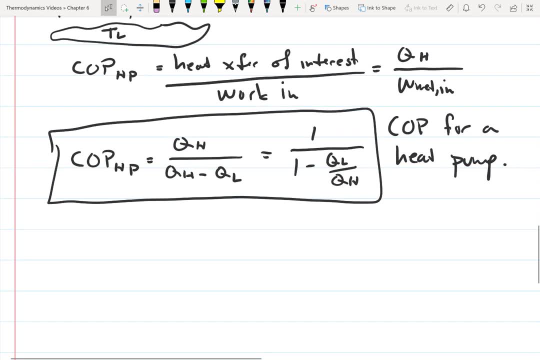 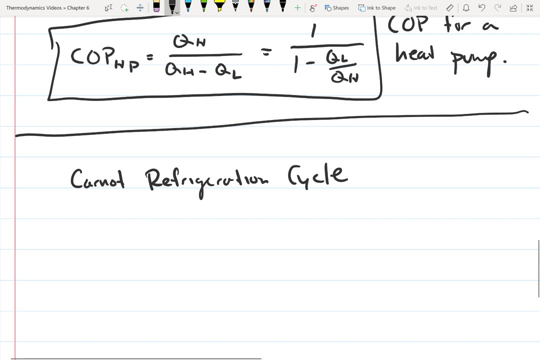 thing with the refrigeration cycle so we can calculate the highest possible coefficient of performance that we can have, and so that's going to be the Carnot refrigeration cycle and this is going to be- and I'm not going to go into as much detail- with the Carnot refrigeration. 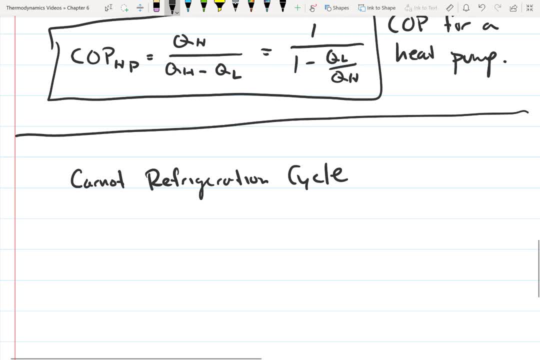 cycle, as I did with the, with the heat engine cycle, because it's the same sort of idea. so remember, with the, the heat engine cycle, the. so the Carnot heat engine cycle was reversible. and it was reversible because everything, every single process in the heat engine was done in a special kind of way that made every process 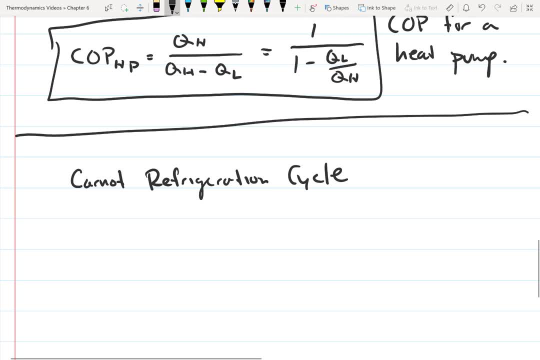 reversible and ideal, and so it led to the highest efficiency that you could possibly have for the heat engine. We can do the same thing with the Carnot refrigeration cycle. We can say that every process in the Carnot refrigeration cycle is ideal and reversible. From that we can calculate. 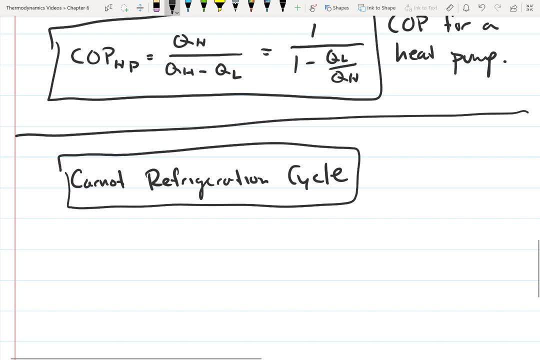 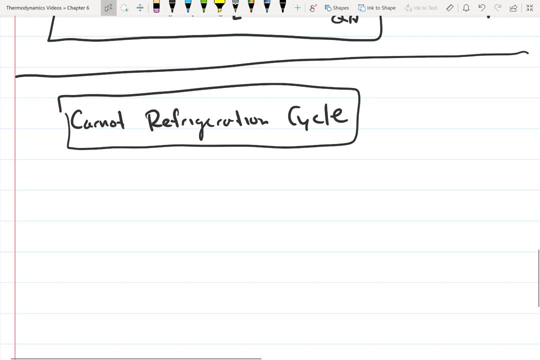 the highest possible coefficient of performance for our refrigeration cycle. So what I'm going to do is write down. so let's just summarize our coefficient of performance. So the coefficient of performance for the refrigeration cycle was 1 over QH over QL, minus 1,. 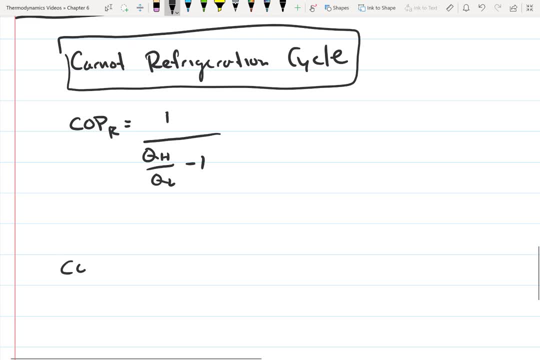 and the coefficient of performance for a heat pump is equal to one over one, minus q l over q h. so what we can do is we can, if we want, to calculate the, so if we want. so, if we're going to say, okay, this is for the carnal refrigeration cycle, we can replace. 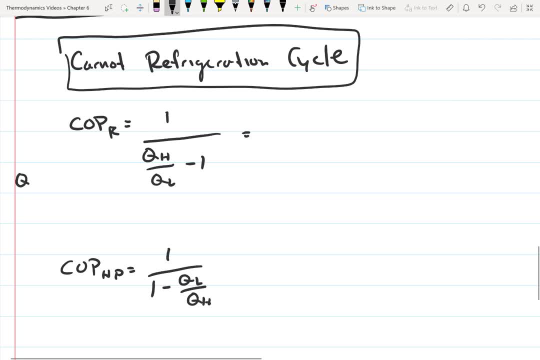 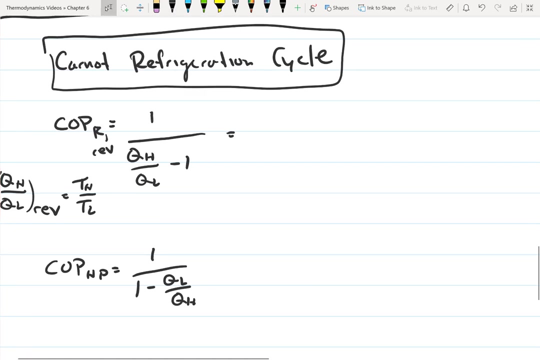 q h over q l, with t h over t l. so remember: q h over q l for a reversible process, for a reversible cycle, is equal to t h over t l. so what we can do is we can say: okay, coefficient of performance for a reversible cycle or for the carnal. 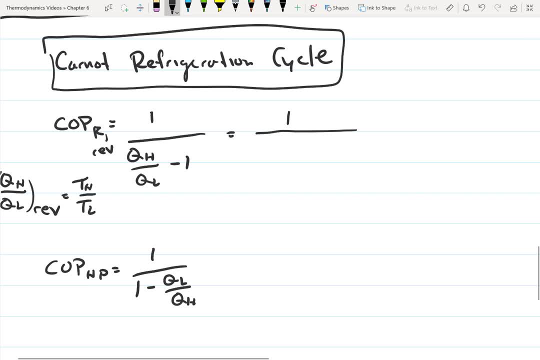 refrigeration cycle is one over, and then this is going to be t h over t l minus one, and for the heat pump, this is going to be one over one, minus t l over t h. so remember for the, for the coefficient of performance. we calculate the coefficient of performance by: 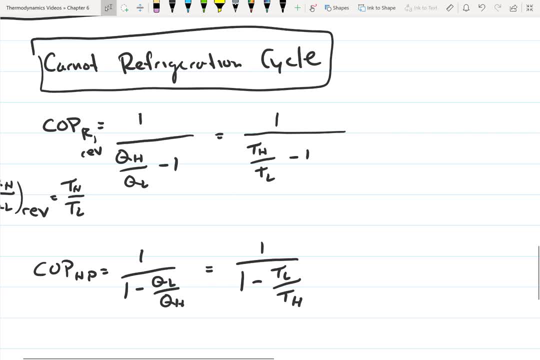 saying: okay, well, what is what are? what heat are we interested in moving? so for the refrigerator, that was q l, so it's the amount of heat that we're removing from the refrigerator. so let's rewrite this. so the coefficient of performance for a refrigerator was equal to q l over the required work. 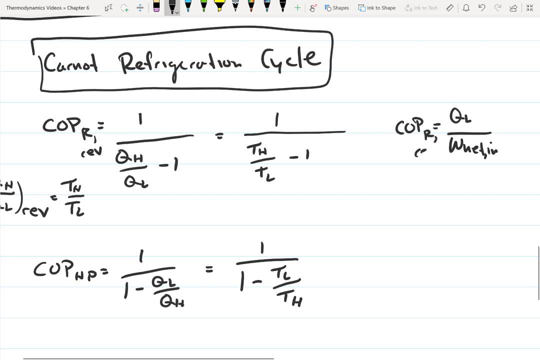 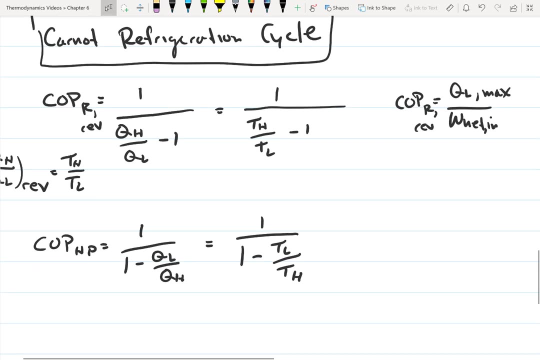 and so for the, for the carnal refrigeration process or the reversible process, this is the maximum heat that we can remove from the refrigerated space for the particular work that we're putting into this refrigerator. and then this is the the same thing with the heat pump. so we 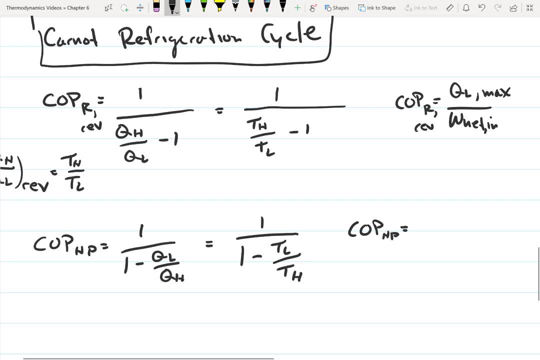 have. so the coefficient of performance for the heat pump for the heat that we're interested in for the heat pump is the heat that's being transferred into the house. so this is going to be q? h over the work net. so the minimum amount of work and if we're considering the heat pump for the carno cycle, we're going to 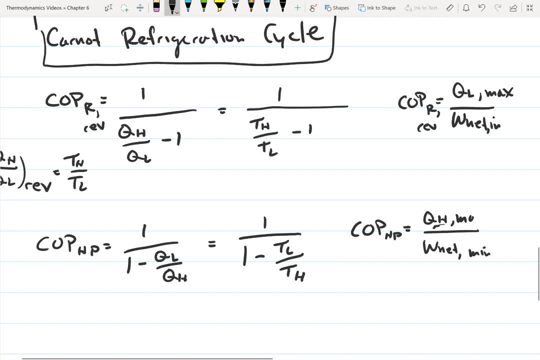 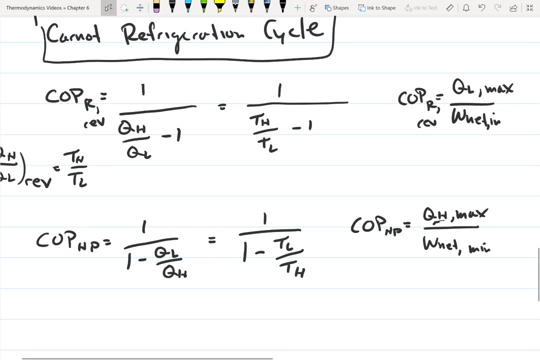 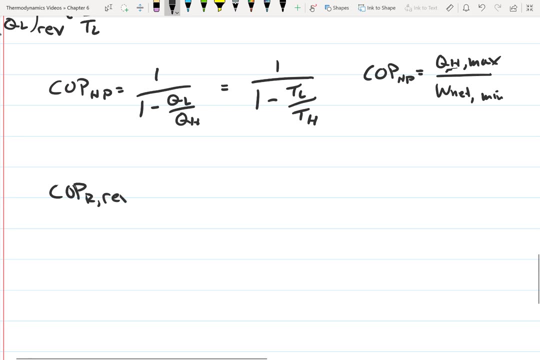 be the maximum heat that we can transfer into the house with the work that we're with, that we're putting into the system. so another way of putting this is: let's so we have our coefficient of performance for the refrigerator this reversible. this is equal to one over t high, over t low, minus one. 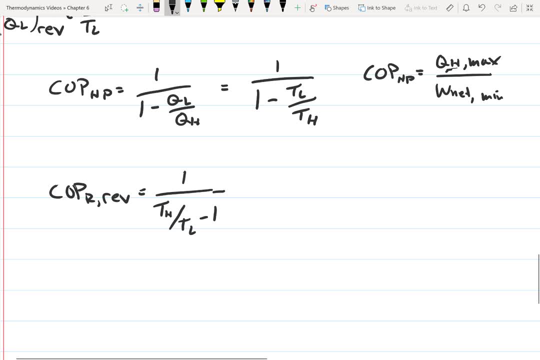 and then we have our coefficient of performance for the heat pump. this reversible. so we have our coefficient of performance for the heat pump. This is reversible. This is equal to 1 over 1 minus T low over T- high. So these are basically the highest coefficients of performance that we can have for a refrigerator or heat pump that's operating between these two temperatures. 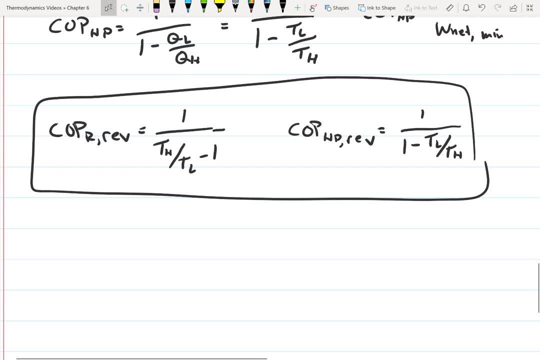 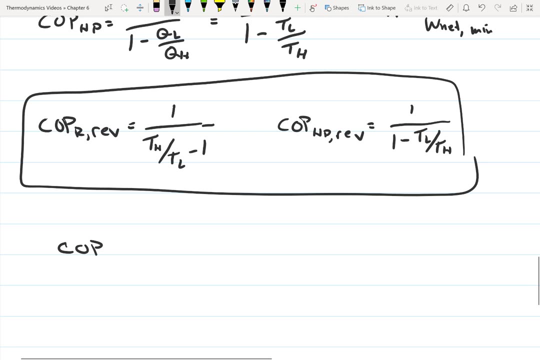 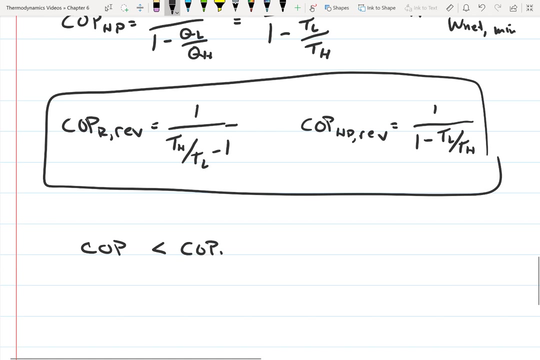 So a real refrigerator or heat pump is going to have a coefficient of performance that's less. So let's say we calculate the coefficient of performance for our actual system. If the coefficient of performance is less than the coefficient of performance for the reversible refrigeration cycle, 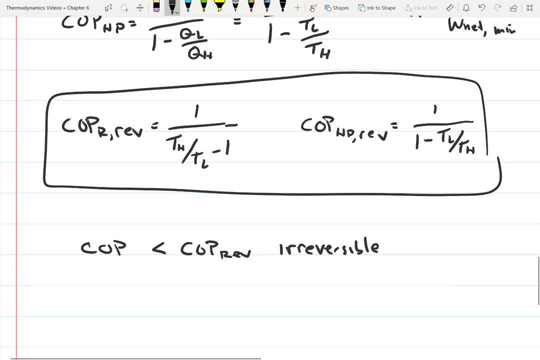 then we calculate the coefficient of performance for the reversible refrigeration cycle. We know this is irreversible. If our coefficient of performance is equal to the coefficient of performance for a reversible refrigeration cycle, we know that this is reversible. And if our coefficient of performance is greater than the coefficient of performance for a refrigeration cycle, 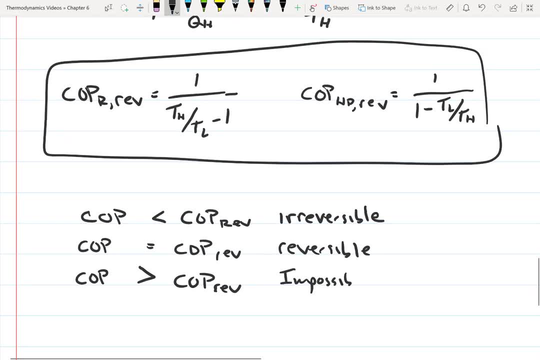 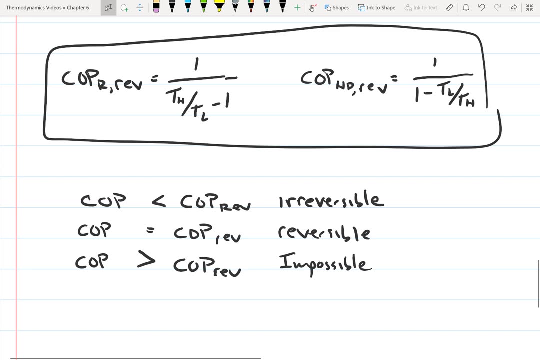 we know that this is impossible. So that means that this refrigerator, refrigerator or heat pump is going to violate the second law and it's not possible. So, basically, we're going to be using the same method to figure out if our refrigeration cycle can work or if it violates the second law, by first calculating the coefficient of 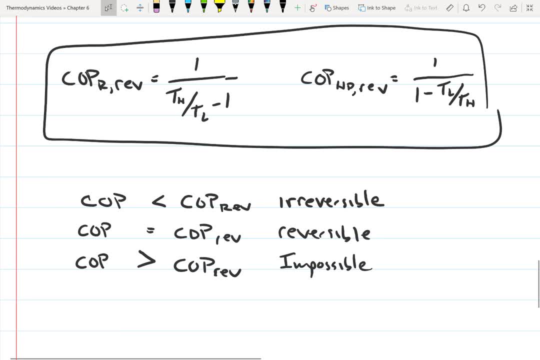 performance for our proposed refrigeration cycle and then we're going to, or for the heat pump cycle. then we'll calculate the coefficient of performance for the Carnot or reversible refrigeration cycle or heat pump and then we're going to compare them and we can determine if our refrigeration or heat pump cycle violates the second law. or if it's going to be possible.